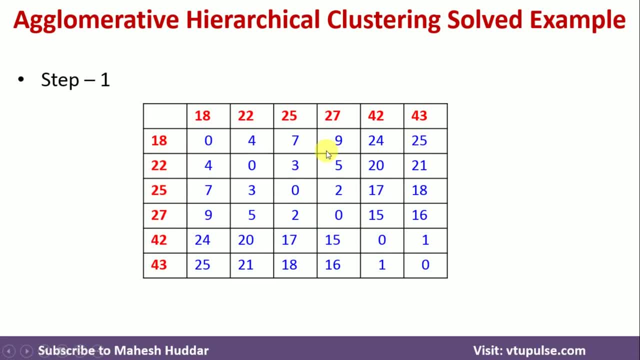 we will get this particular matrix. so, once you get this particular matrix, we have to clearly observe this particular matrix and we need to find out the distance, or the minimum distance between the two data points. if you look at this particular, the distance matrix, this one, that is, the distance between 42 and 43, is 1, which is the minimum among all these things. 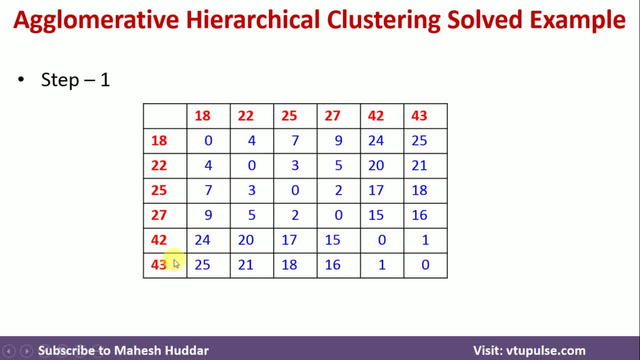 so what we do here is we will merge this particular 43 to 42. the meaning is we will create a cluster consisting of 42 and 43 at the first step. so this is these are the two points, that is, 42 and 43, which is indicated here. they have the minimum. 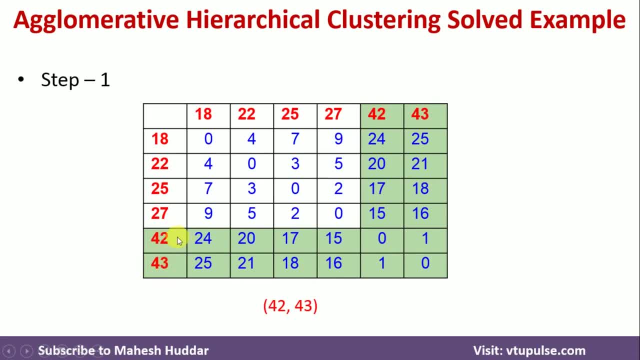 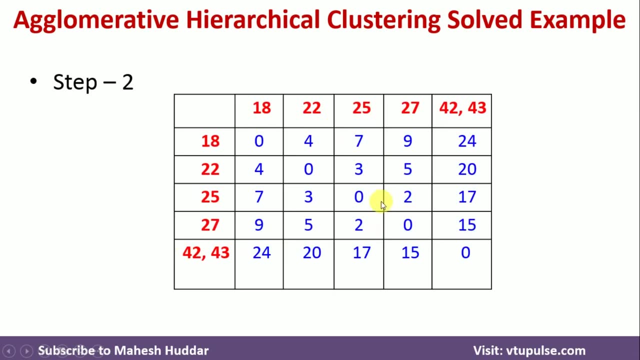 distance. so we will merge this 42, 43 into 42 here. so it looks something like this: so what we do here is we will remove this particular row and column of what we can say, that 43 and 43 will be merged into 42 here. so that is. after doing that, this is how actually the matrix looks like. 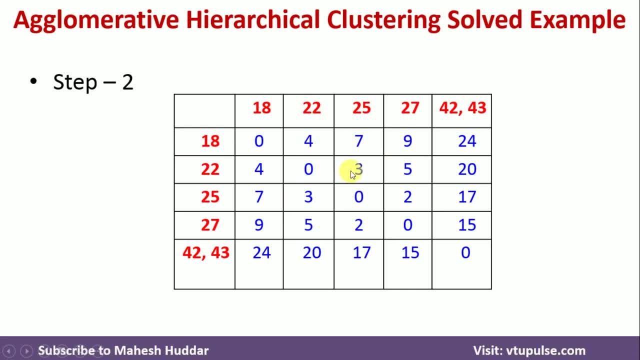 now from this particular matrix. in the second step what we do is we will try to find the minimum distance again. now if you look at this particular matrix closely again, you can see here the distance between 27 and 25. that is the minimum here. so what we do in this 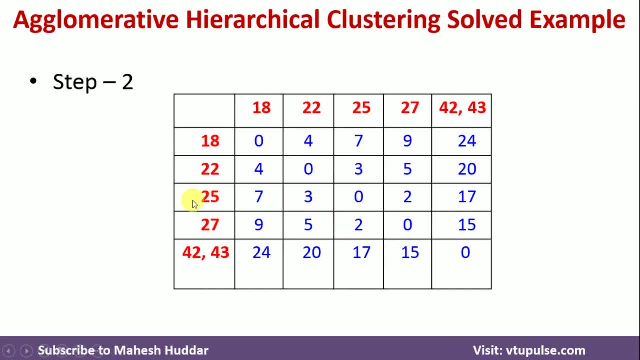 case is we will merge this 27 into 25, we will create another cluster and then this particular 27 row and column will be removed in this case. so this is how actually we can show it with the help of pictorial representation: 27 will be merged in 25. 27th row and column will be removed in this case. 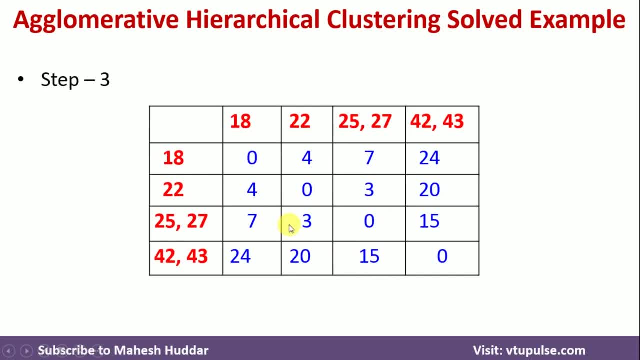 after that, we will get something like this now from the remaining data points. what we need to do is we need to again find the minimum distance. if you look at this particular matrix, the distance between 20 to 25- 27 is minimum, because that is 3 here. so we merge this 25 and 27 into 22. 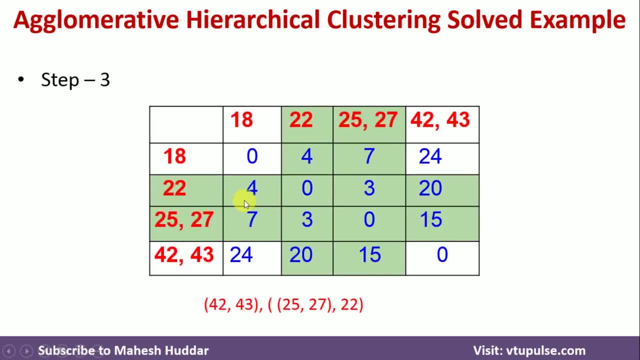 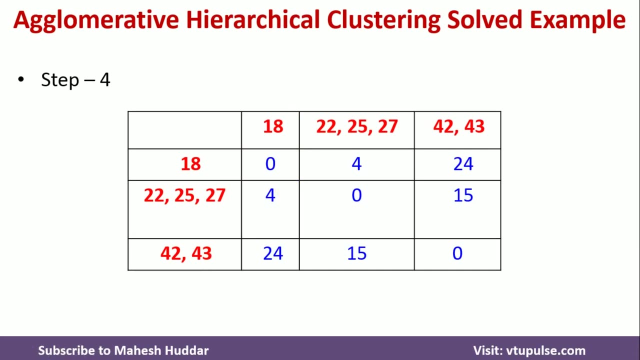 and then this row and column will be removed in this case. so that is what i have shown over here, and once i merge it it will become 25, 27 already we have merged it to this one. we will merge 22 in this case. so after doing that, we will get this particular, the resulting matrix, here now.